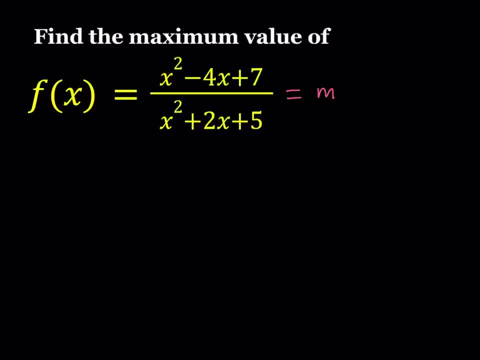 and basically to find the maximum value of f, of x. if I find the maximum value of m, then I'll be done. So let's go ahead and cross, multiply both sides and we should be getting x squared minus 4x plus 7 is equal to mx squared plus 2mx. 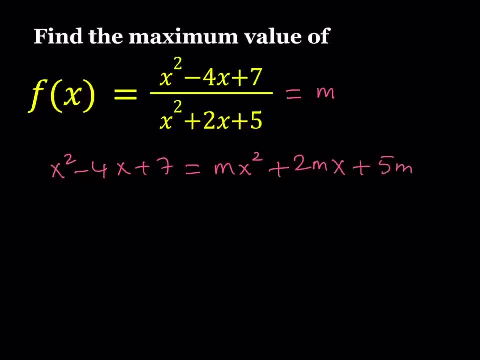 plus 5m. Okay, I'd like to put everything on the same side. so mx squared minus x squared, so it's going to be m minus 1x squared, and then 2m plus 4x, and then finally, 5m minus 7 is equal to 0.. 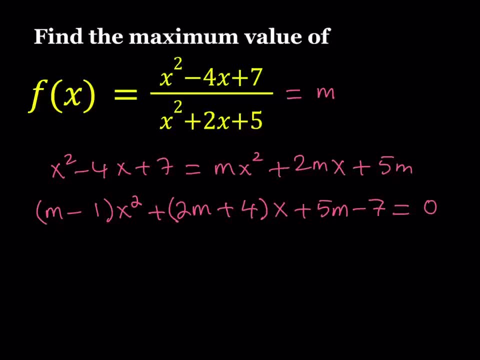 Okay, now we're trying to find the maximum value of m, and we got a quadratic equation in x, but the coefficients are in terms of m, So I want this function to have real values, obviously, otherwise we can't really find the maximum or minimum value. So what we're going to do here is: 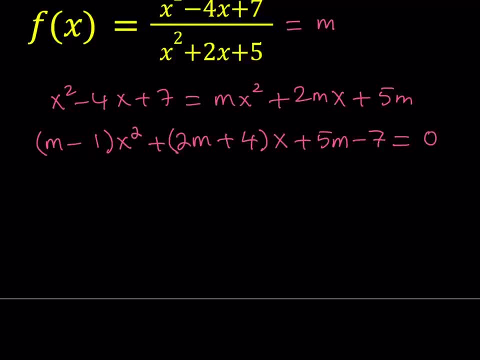 we're going to be looking for real values of x, and how is that possible? We're going to be looking at the discriminant of this equation. So let's go ahead and write the discriminant. The discriminant of this quadratic equation is going to be b squared. The discriminant is delta. 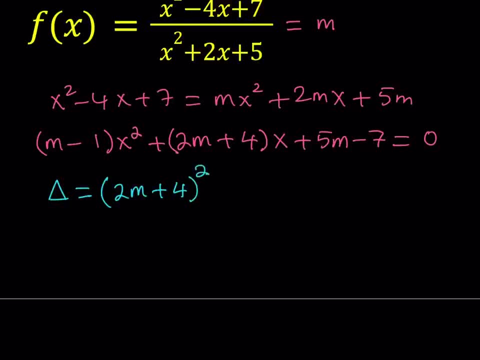 I'm using the correct letter here. So b squared minus 4ac. Okay, c is the constant. Okay, now let's go ahead and calculate this delta. Let's simplify as much as possible. This is going to be 4m squared plus 16m plus 16, and then this: 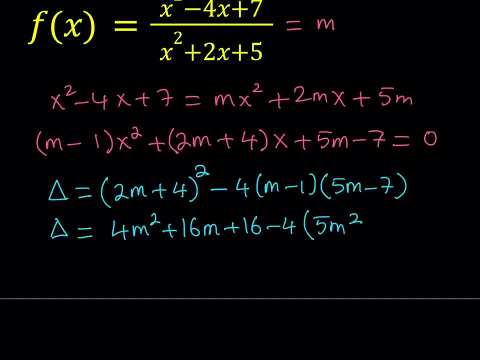 is going to be negative 4 times the quantity 5m squared. So I should be getting negative 7m and negative 5m, which is going to give me negative 12m plus 7m. Let's go ahead and distribute this and simplify: 4m squared plus 16m plus 16, and then I get. 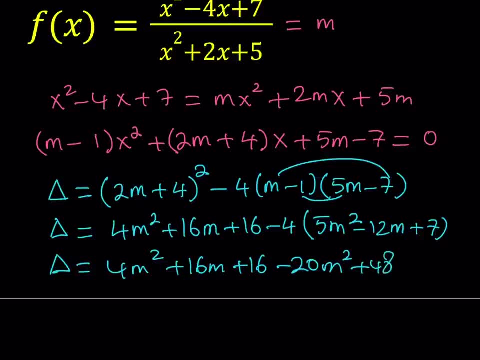 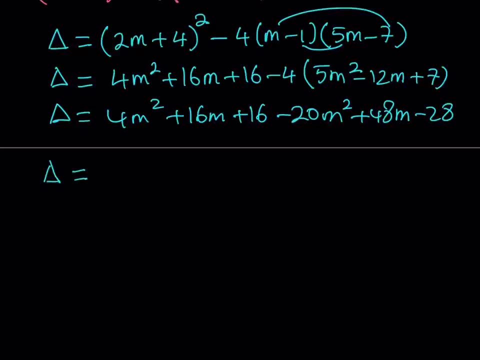 negative: 20m squared plus 48m minus 28.. Let's go ahead and combine like terms and write our equation: or for the discriminant, 4m squared minus 20m squared is negative 16m squared here, and then 16m plus 48m. that should give me. 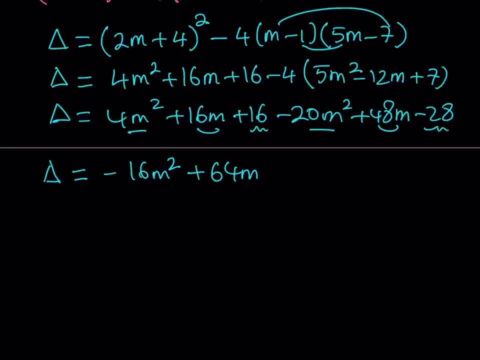 64m and finally, 16 minus 28 should be negative 12.. Okay, now let's simplify this a little bit more. I can take out a common factor in this case, that will be a negative 4, and I want to keep the m squared positive. So negative 4 would be a good one. and this gives me, inside the parentheses: 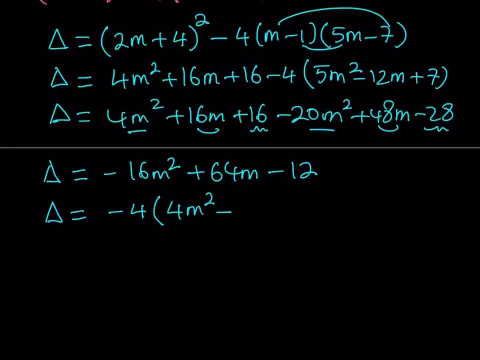 4m squared minus 16m plus 3.. So what am I looking for? I want the real x values for this function, and this is the discriminant right, and I want the discriminant to be non-negative. So in other words, my discriminant needs to be greater or equal to. 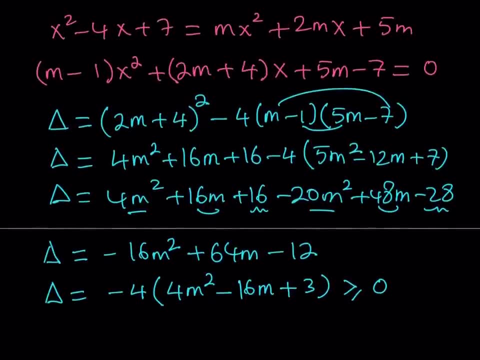 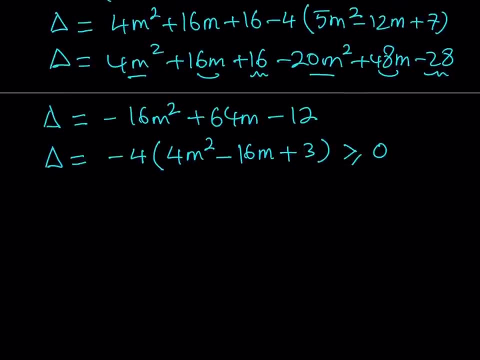 0, so that my quadratic equation is going to have real solutions. Okay, and so we're going to be using this inequality to find the max and min values for m. Now, what is this supposed to mean? Well, we did get a quadratic inequality. So, first of all, to get rid of the negative. 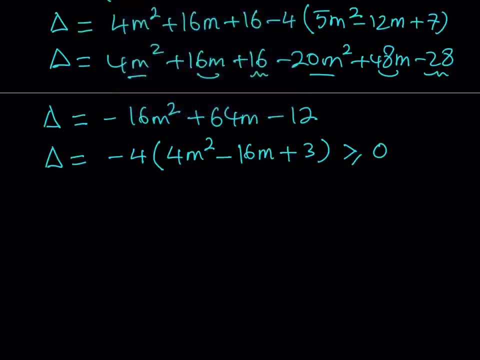 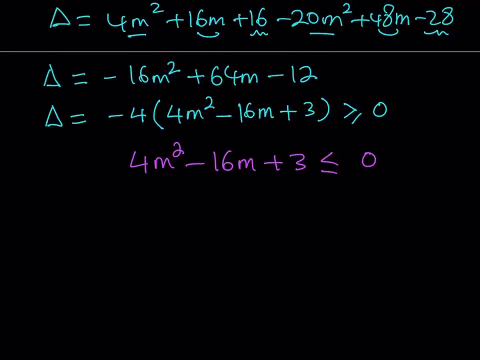 let's go ahead and divide both sides by negative 4, and when you do remember that the inequality sign will be changed. So instead of greater or equal to 0, it's going to be less than or equal to 0.. Now, when you get a quadratic equation like this, basically you're 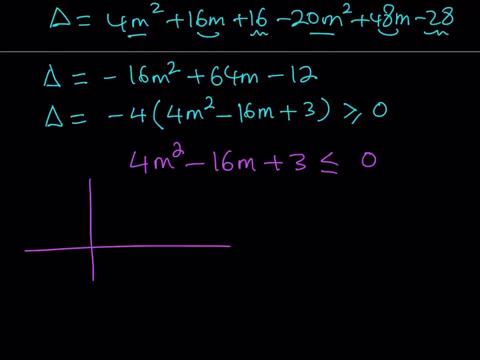 talking about a parabola. Let's talk about this and notice that the sum of the roots is positive. the product of the roots is positive, So you're kind of talking about two positive roots. It doesn't really matter much here, but if you have a quadratic equation, 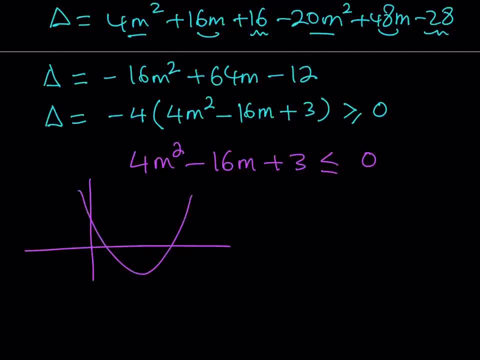 right like this. So you have a parabola and you want this parabola, the y values, to be less than or equal to 0. You're basically talking about being between the roots here. So if this is m1, 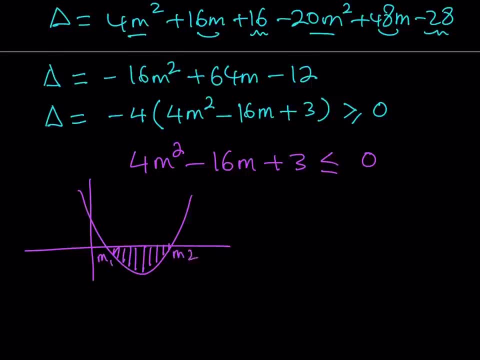 and this is m2. you have to have your m values needs to be in that interval so that this expression here is going to be less than or equal to 0.. So that's what we're going to do. So let's go ahead and find the roots first: m1 and m2.. To find m1 and m2, you're going to have to find the roots. So 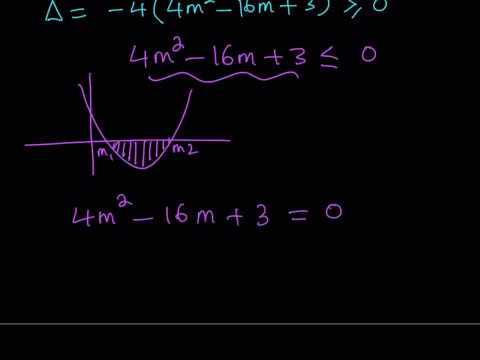 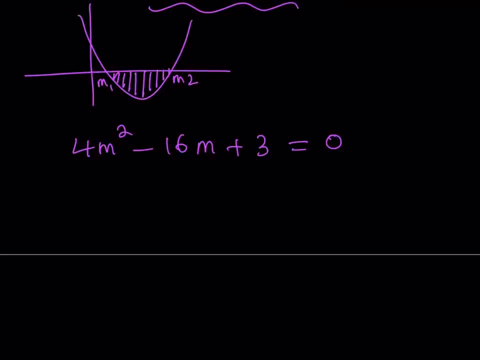 we're going to solve this as a quadratic equation, So it's kind of like a quadratic within a quadratic, All right. So to be able to solve this, I can use the quadratic formula, and the quadratic formula tells me: m values are negative, b plus minus the square root of b squared, which is 256. 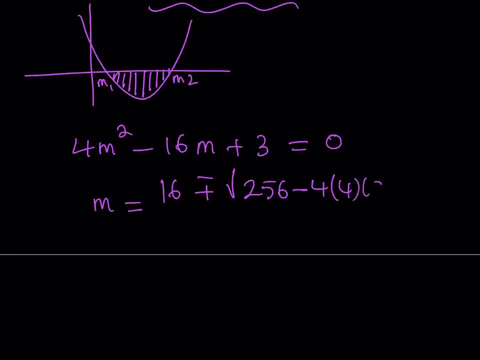 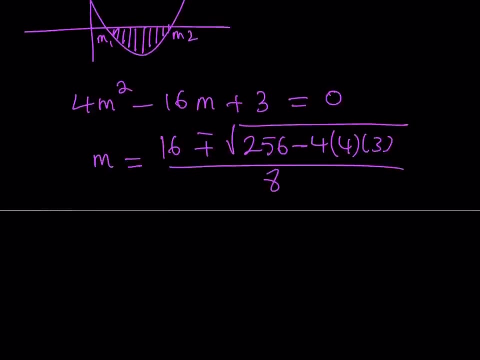 minus 4 times a times c. Now, obviously, to make it a little easier on ourselves- and this is going to be 2a- We can just factor out a 16 here, obviously, because 256 is divisible by 16. And 4 times 4 is 16. So I can easily plot a 16, which means I'm going to get a 4 outside the 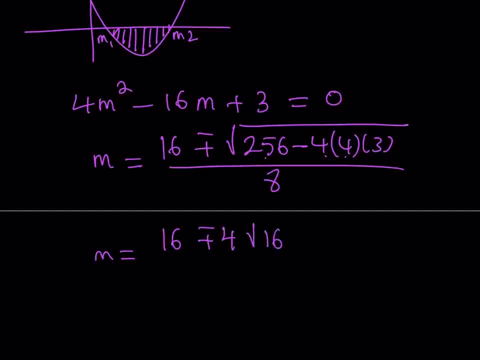 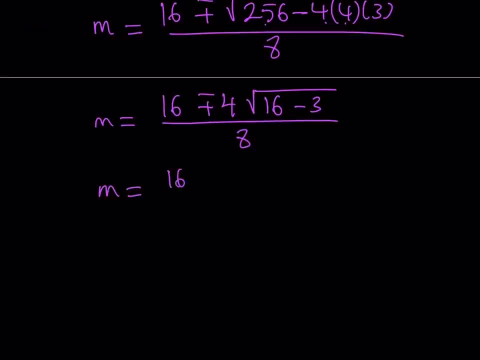 radical And inside, since we divided by 16, this should be a 16 and this should be a 3.. That means that my m values are going to look like this: 16 plus minus 4 times the square root of 13, all over 8.. Obviously, this can be simplified because there's a common factor: Everything can 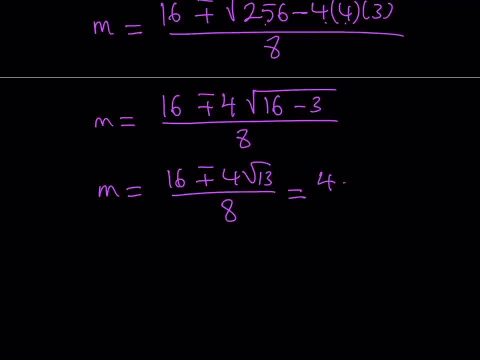 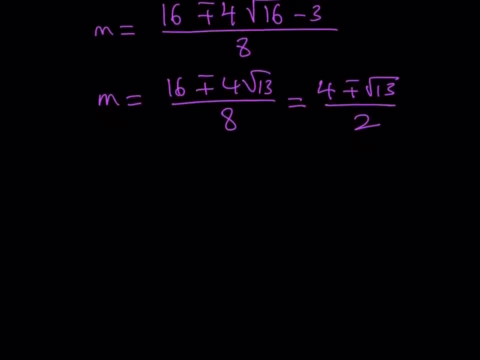 be divided by 4.. If you do that, you get 4 plus minus root of 13 divided by 2.. So these are the m values. Let's go ahead and write them down separately. So m1- the smaller value, is going to be this one and the larger m value is going to be this one. 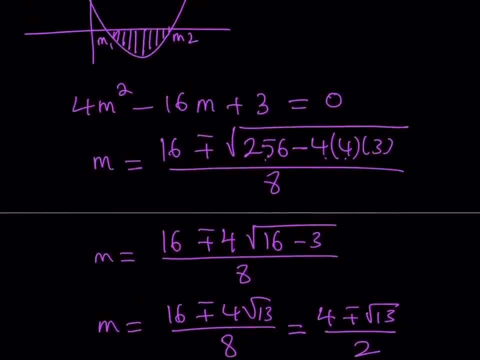 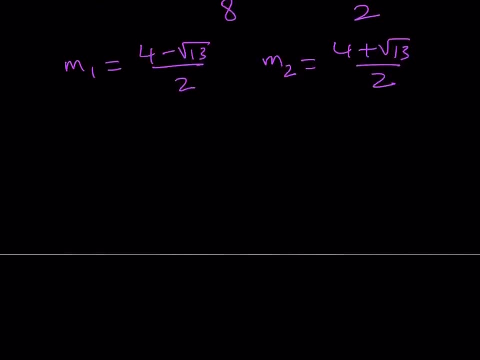 And, as I said earlier, if you want this quadratic to get negative or less than or equal to 0 values, non-positive values, then you're you have to be between m1 and m2.. So you want m to be between these two values. Let's go ahead and write it down. 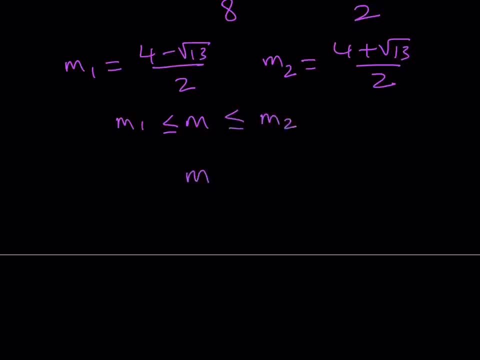 First of all, I can write it like this, and then just replace m1 with 4 minus root 13 over 2, and this one with 4 plus root 13 over 2.. Great, Now remember we were looking for the maximum value of f of x, which was equivalent to the maximum value of m, And here we did find it actually. 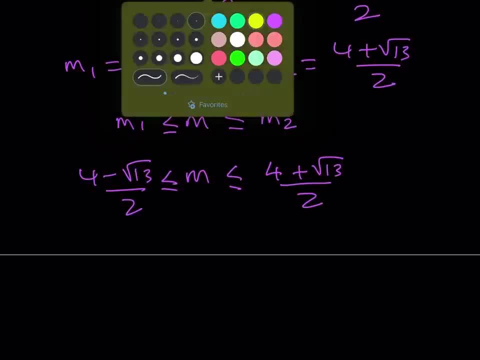 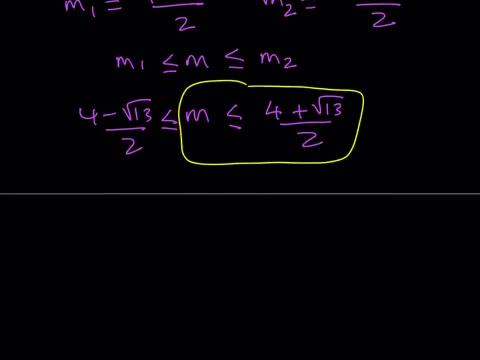 because we know that m is less than or equal to this value here, and this tells us the maximum value, because m cannot be greater than this value. So we can write it like this. So we can write it: so, basically, maximum f of X, which is the same as maximum M, is going to equal 4. 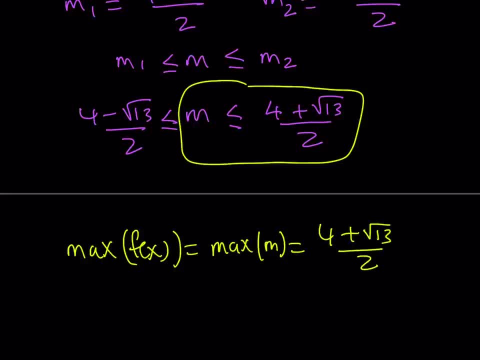 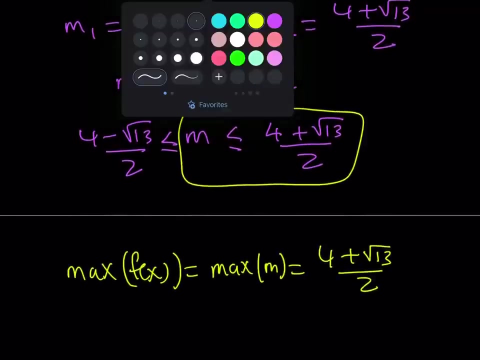 plus root 13 over 2. notice that with this method we did not have to find the X value which makes the function take a positive value. we directly found a maximum value. and also it's an algebraic approach as opposed to a calculus approach- not that I don't like calculus, but it's just an alternative. so this: